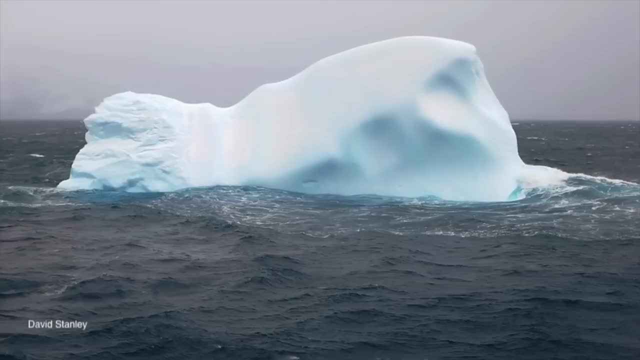 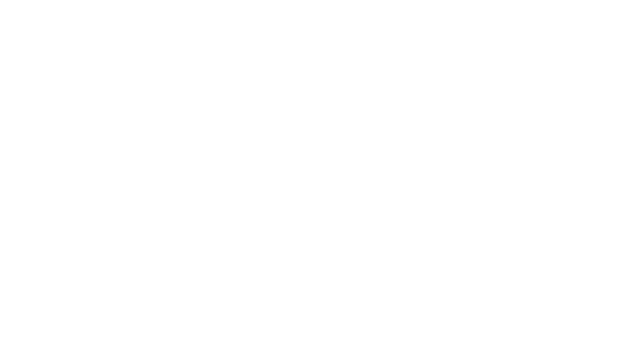 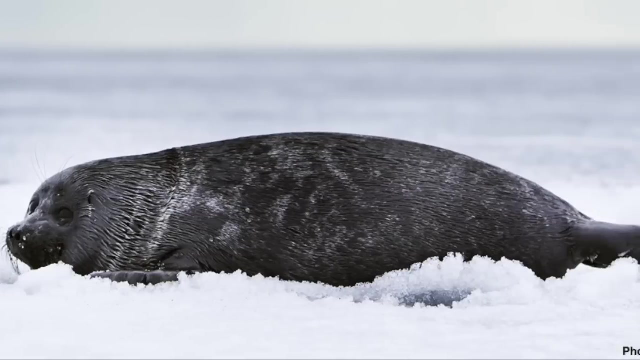 seem to have colonized their homeland in the late Pliocene, before any evidence of a massive ice-dammed lake. Yet the Peritethes was also long gone by this time. The genetic evidence doesn't match up with any large, deep watery pathway into the interior. So did the ancestors. 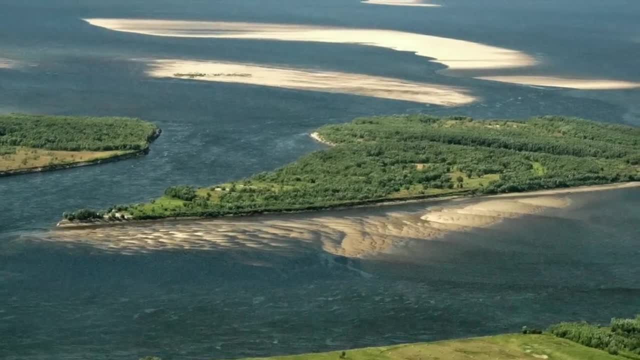 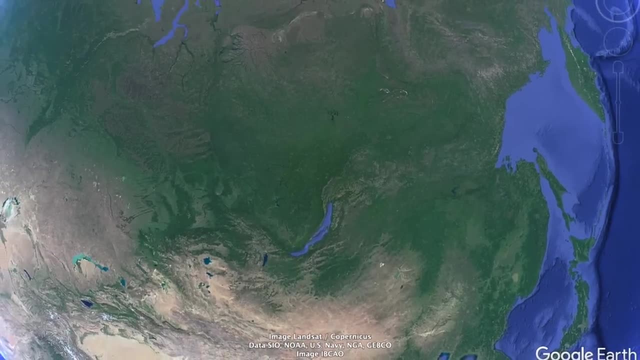 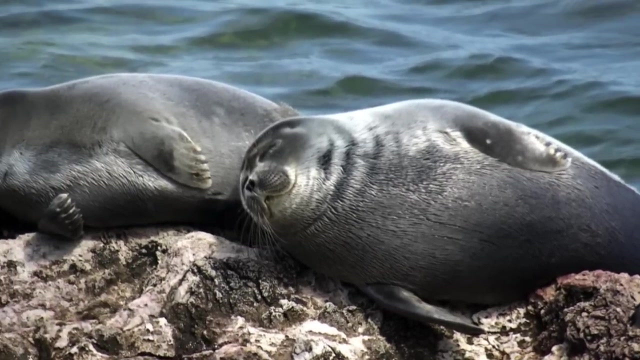 of a Baikal seal use nothing but rivers to reach the center of the Asian continent? Could seals really swim over a thousand miles upriver to a new homeland? Is this an important, entirely ridiculous notion? Well, I can understand why you might think so, but I would argue it's not. out of the question. According to some historical records, harbor seals were regular visitors to Lake Ontario and Lake Champlain before 18th century. hunting pressure wiped them out. If it weren't for Niagara Falls, those seals might have been able to colonize the Great Lakes. And in modern times, Baikal seals have been sighted 400 kilometers downstream from the lake in the Angara River. But it isn't just the distance that makes this journey so surprising. Today, the river draining Lake Baikal has several rapids. 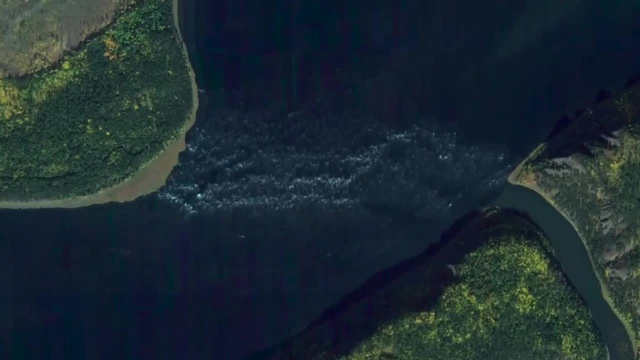 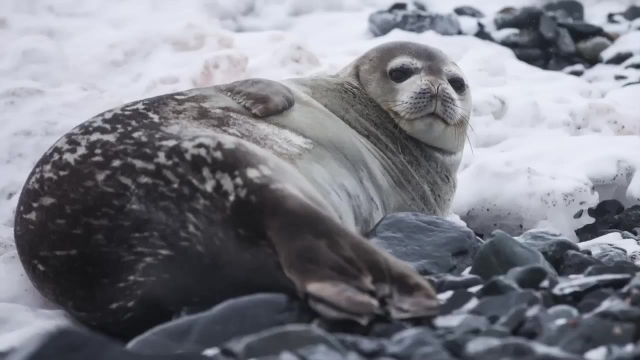 and the topography wouldn't have been all that different in the late Pliocene. Is it hard to imagine a group of seals hopping around multiple series of rapids on their long journey into the hinterland without being picked off by predators? Again, I can understand why. 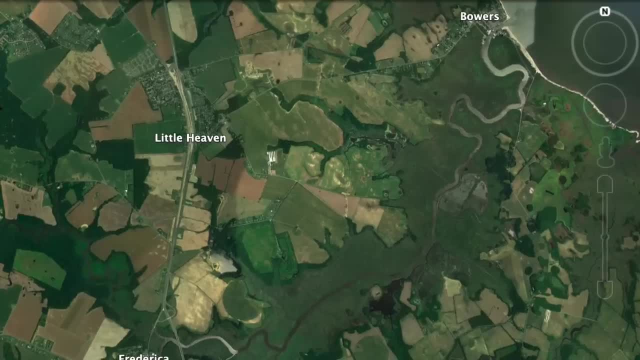 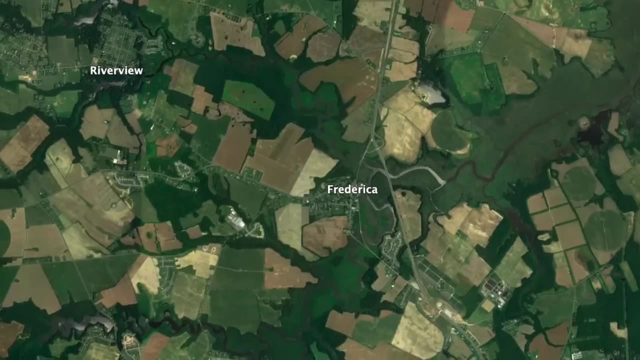 But consider this story out of Delaware from 2017.. In the winter 2017, year, a harbor seal entered a small creek that emptied into the Atlantic. He swam past oak trees and old barns until about 10 miles inland he reached a spillway. 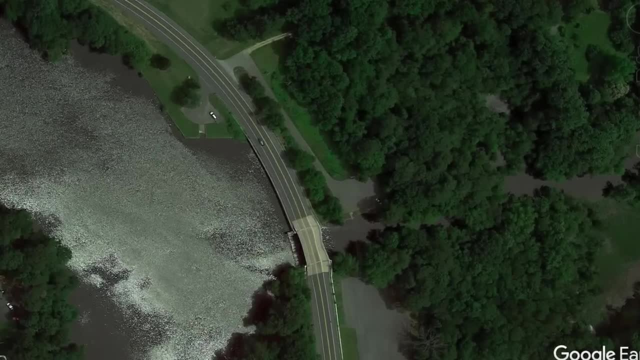 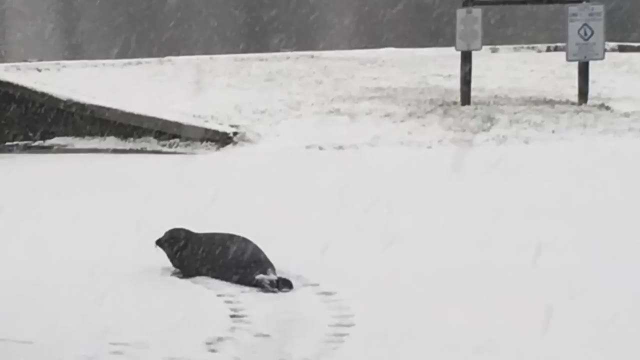 But instead of turning around, he just hopped out into the adjacent parking lot, hopped about a hundred yards up the driveway to the main road, hopped across the main road into the next parking lot and slid down the boat ramp into the. 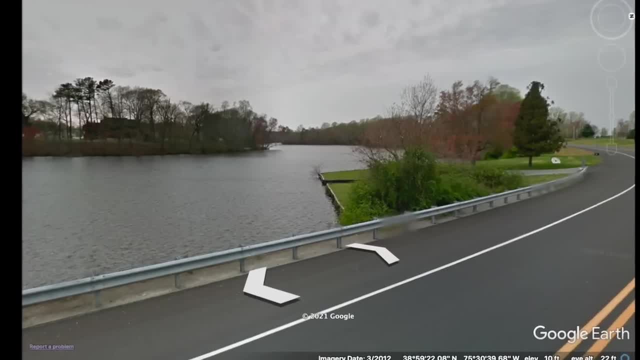 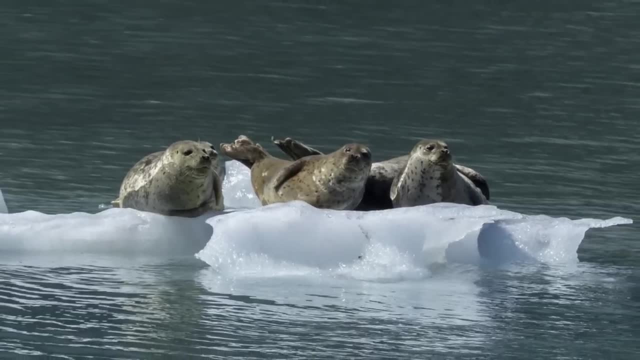 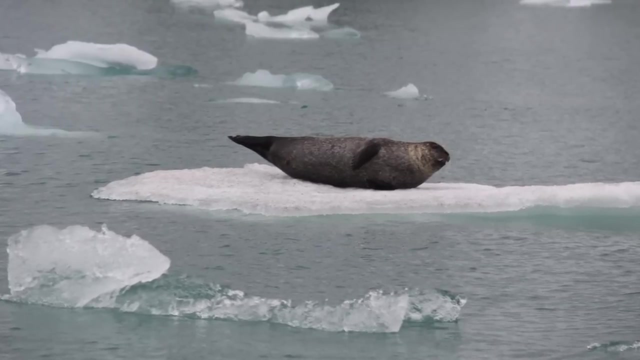 pond above the spillway. There he spent a few months happily eating sunfish and bass before wildlife experts moved him in the spring. This might just seem like fun trivia, but I do think it says something more broadly about seals: That we shouldn't underestimate their inquisitive nature or drive to explore. 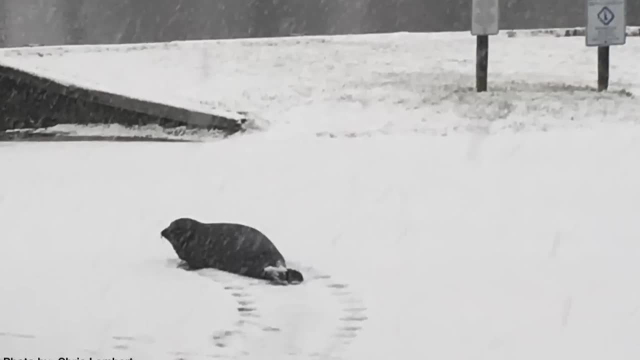 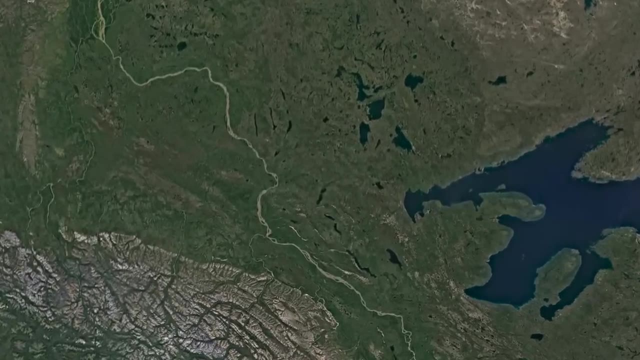 and find new resources. We humans were there to witness this seals journey because it happened in a more populated area. In the more sparsely populated far north, seals might swim upriver and hop around obstacles more often than we expect. However, those brave seals reached. 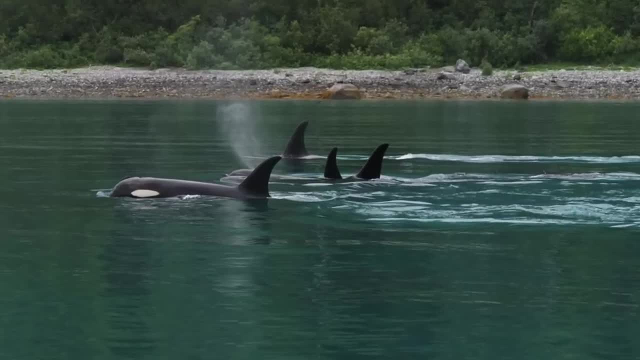 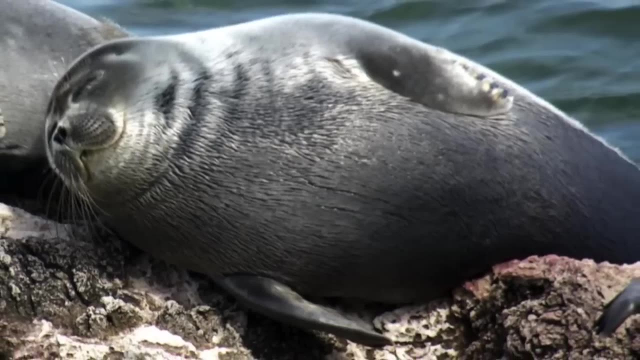 Lake Baikal. their gamble clearly paid off. Today, their ancestors can swim and eat without worrying about orcas or Greenland sharks lurking in the shadows. Not a bad deal for a humble seal. Thanks for watching.